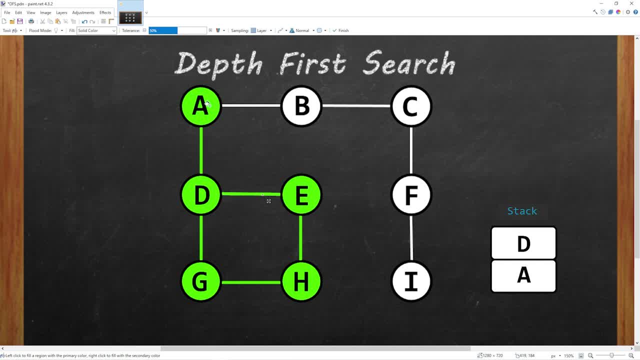 So we will pop all of these nodes off of the stack all the way back to A, which has unvisited adjacent neighbors, and this time we will go down this route and push all of these nodes onto our stack And we have reached the end, Using a death first search approach to navigate this graph. 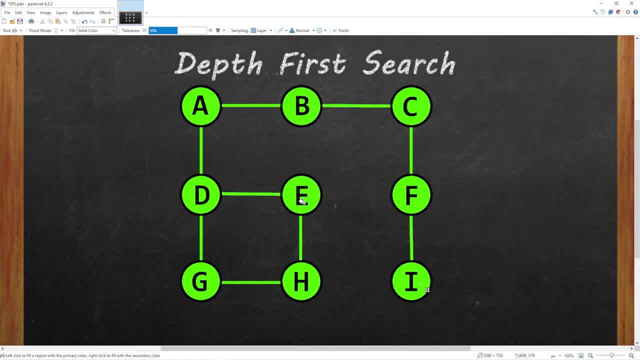 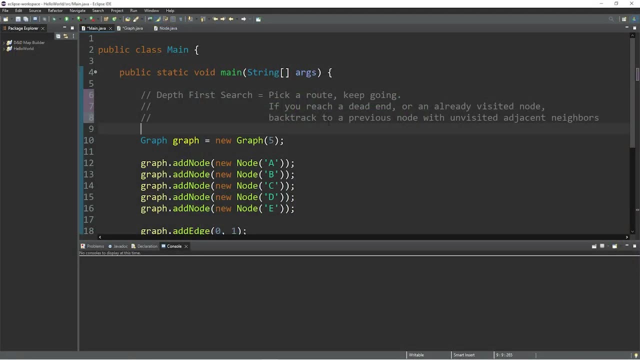 when simplified, you pick a route, you keep going. when you reach a dead end or a node you already visited, you backtrack to a node that has unvisited adjacent neighbors and you repeat steps one through two. All right, well, let's implement this in code now. And here we are people. So I'm going. 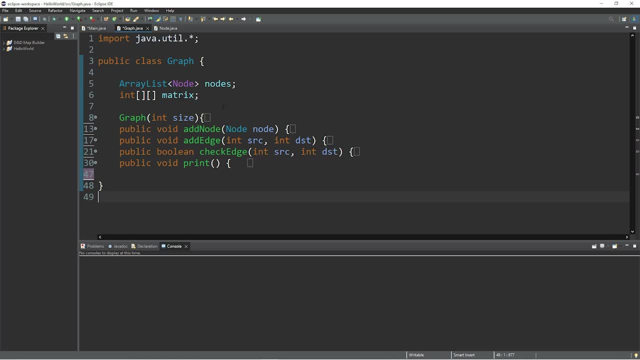 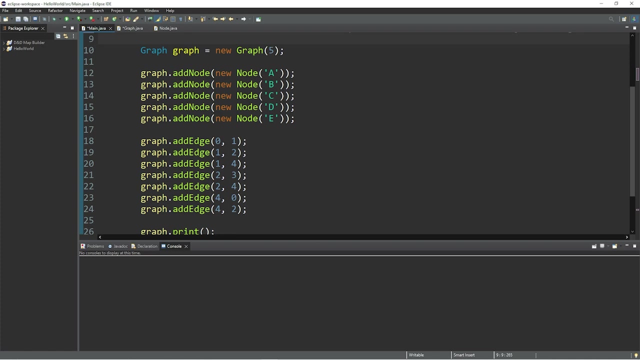 to be using a graph that utilizes an adjacency matrix. If you're using an adjacency list, the code's just going to be a little bit different, but the concept is really still the same. I'm using a graph that utilizes an adjacency matrix. So in the previous videos we have a node class, a graph. 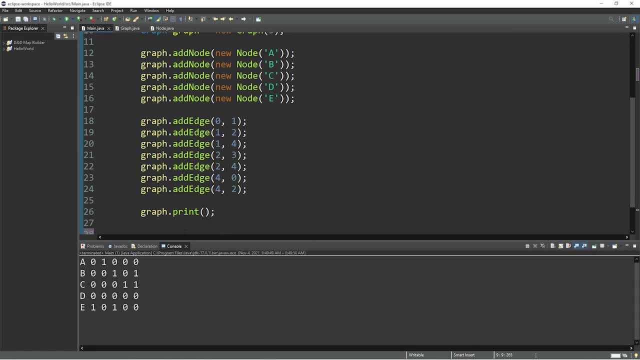 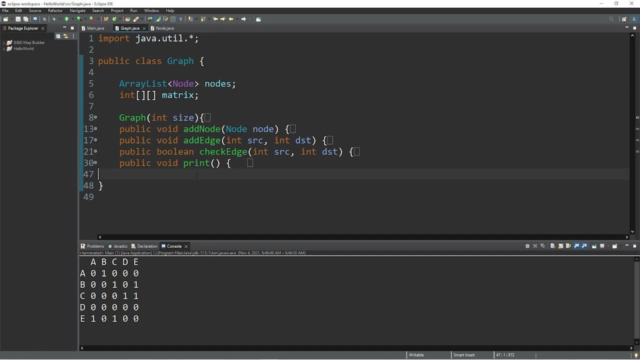 class and in the previous videos we've already populated this graph with nodes and edges, And then I'm just going to print this: This is my adjacency matrix. Now, within the graph class, we're going to create a depth first search method and a helper method, So this will be public void. 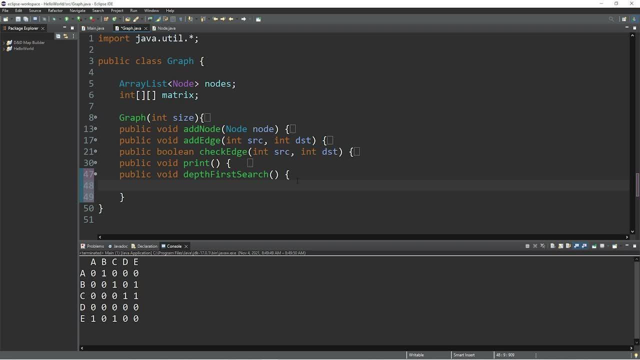 and we will name this depth first search And there will be one parameter, an index of where we want to mark the nodes that we've already visited. What some people like to do is that they will create a Boolean within their node class, such as Boolean visited, and they'll just mark it as false. 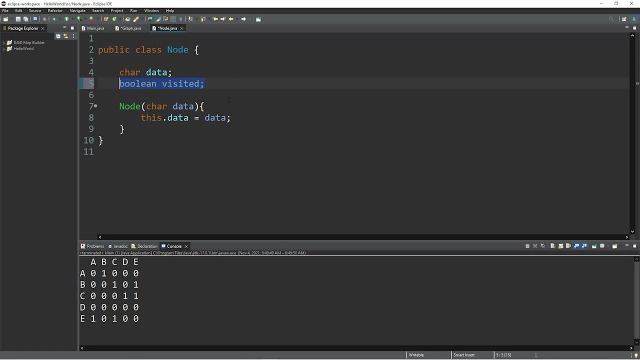 or true. However, it's very easy to forget to change these back to false when you exit the depth first search. So what I'm going to do instead is create an array of Booleans, and the size will be equal to the length of the matrix. So let's create a Boolean array And I will name this visited. 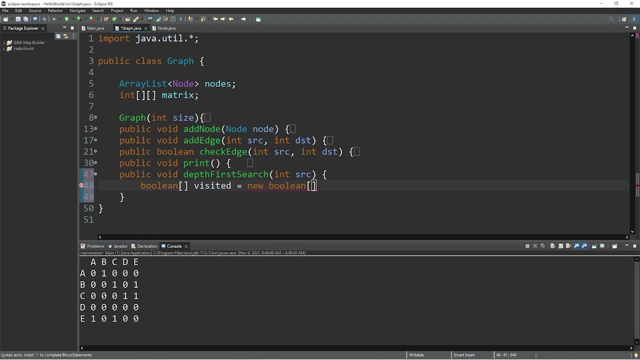 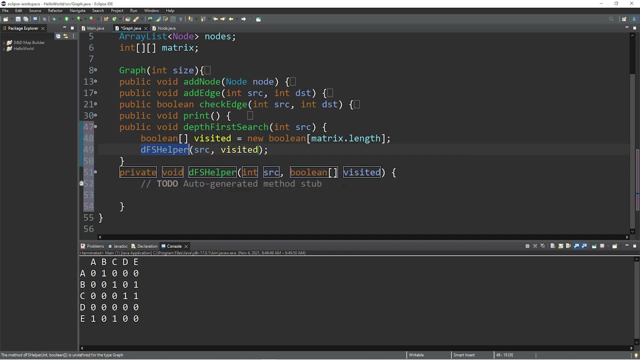 equals new Boolean. The size of our array is the length of our matrix. Then, lastly, we will implement a helper function, So let's name this DFS helper and we will pass in our source and our Boolean array visited. Then we just need to create this method: private void DFS helper, And there are two parameters: int source. 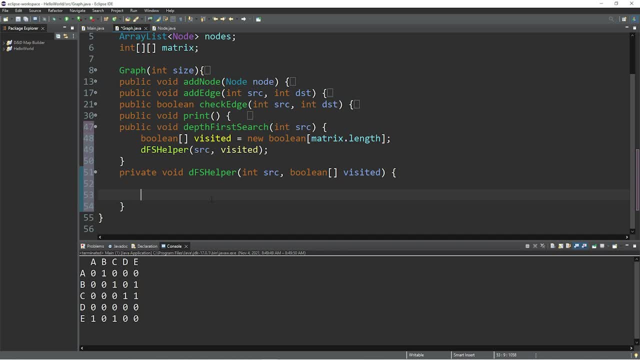 and an array of Booleans named visited. You can either implement a depth first search iteratively using a stack, or you can just create a Boolean array. And we're going to create a Boolean array using a stack, or you can utilize the call stack if you use recursion. In this example, we're going. 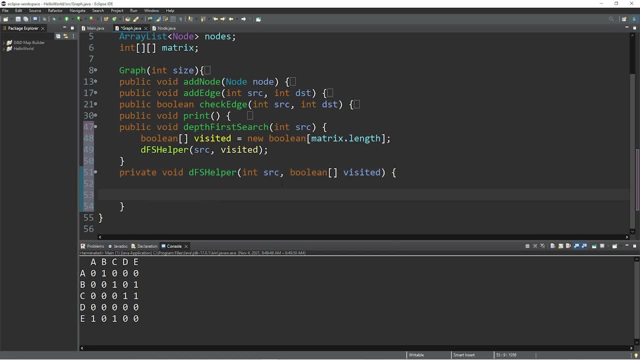 to use recursion. When we invoke this helper function, we're going to check to see if the current node that we're on is visited or not, And we can use an if statement If our visited array at index of source is equal to true. or you could write the shorthand and just say if visited at. 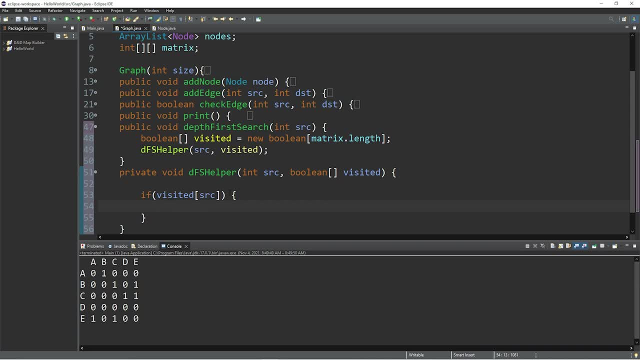 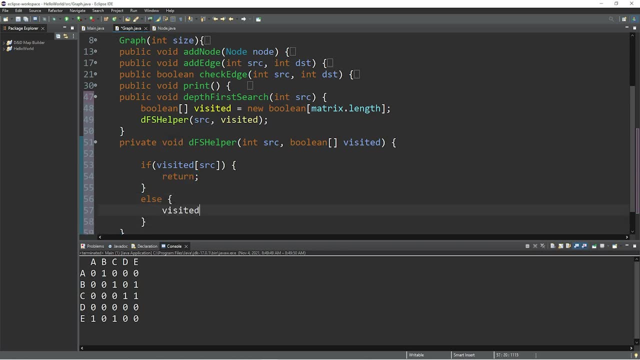 index of source, since this returns a Boolean value. If we've already visited this node, we're going to return, else we will mark this node as visited. Else visited at index of source equals true, If you would like, although this part's not necessary within my console, I'm just going to 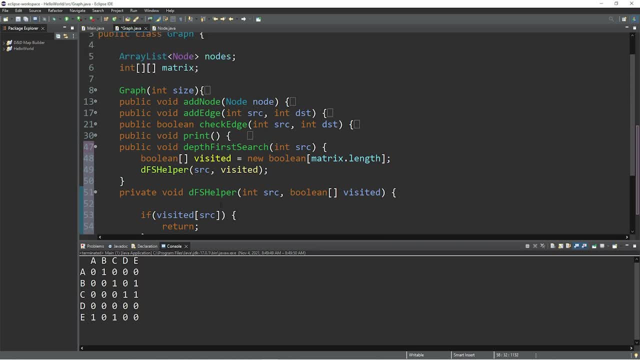 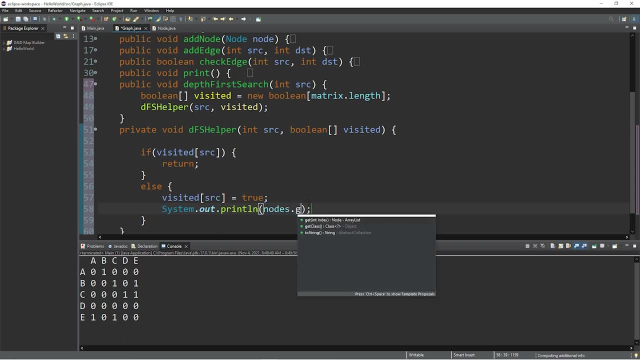 print that we visited this node. So within a print line statement I do have my nodes. within an array list I'm just going to access the data of one of these nodes: dot get source, dot data plus equals visited. This part technically isn't necessary but it's going to help with my 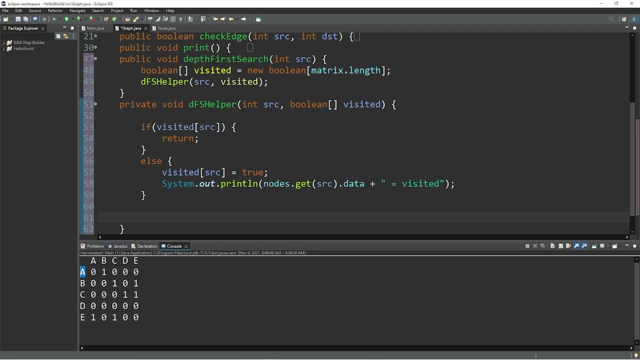 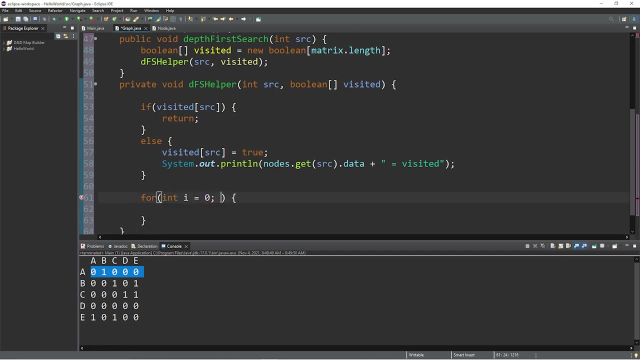 demonstration. In this example. maybe we start at node A. we need to find any adjacent neighbors. if we're using an adjacency matrix, we need to iterate over this row. we can use a for loop for that. So int i equals zero. we will continue this as long as i is less than our matrix at index of. 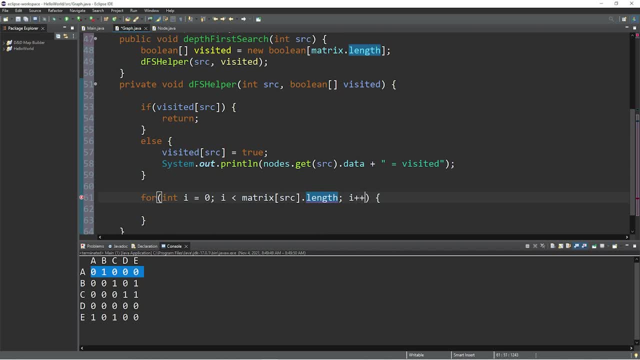 source. This equals the length of a row and then increment i by one. we're checking to see if one of these elements is a one That means that's an adjacent neighbor that we can travel to using an if statement, if matrix at indices of source and I sources, the row that we're working with I is: 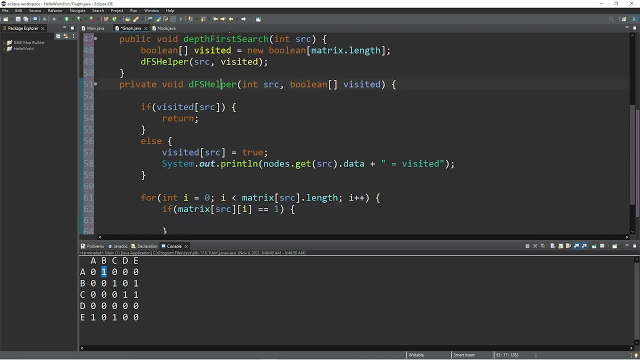 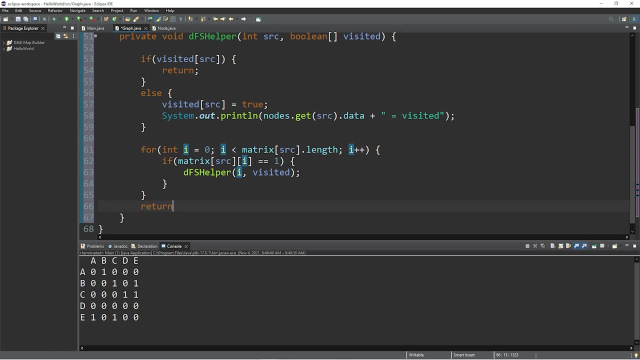 the column. If this is equal to one, then we will invoke the DFS helper method again. So this is recursive. So we're going to pass in i, as well as our Boolean array named visited. if we successfully search through an entire row outside of the for loop, let's return And that's it. So let's run this. 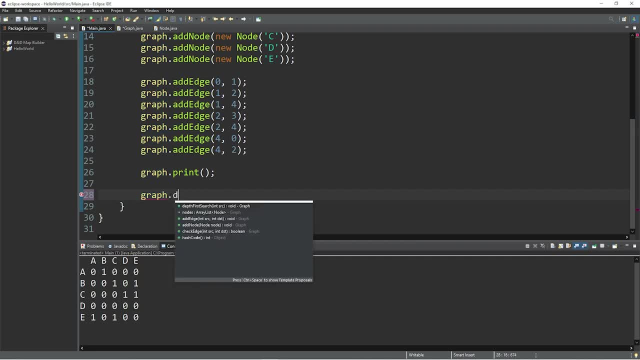 Within my main class, I will call the graphs depth first search method and pass in an index of a starting node. So let's begin at zero. we visit a first, then B, C, D, E. let's try B, which has an. 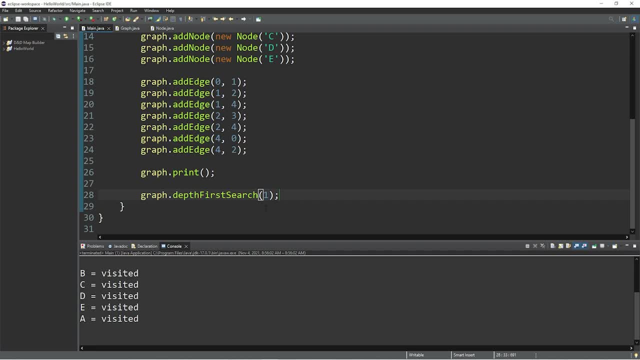 index of one, B C, D, E, A, B C, which has an index of two: C, D, E, A B. Okay now pay attention to this. This is a directed graph and we're beginning at D. there's no place that we can go, So we're stuck at D. we only visit. 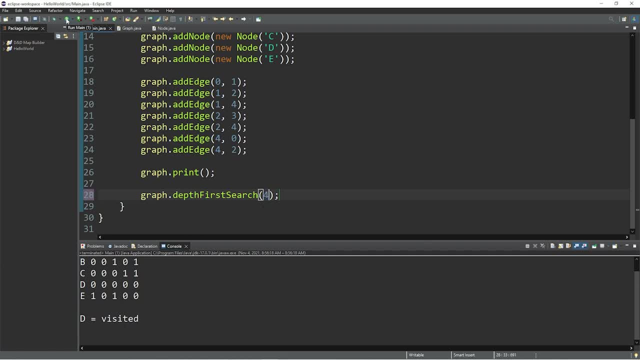 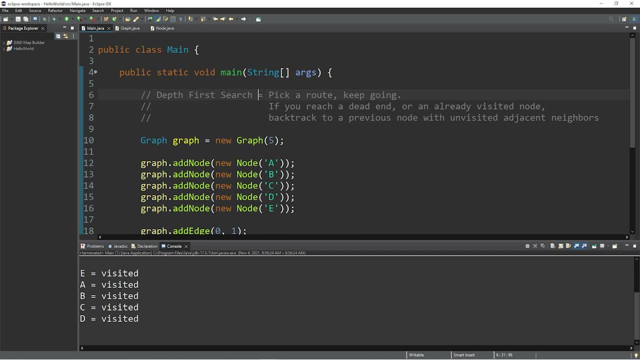 D. And lastly we have E, which has an index of four: E, A, B, C, D. All right, everybody. that is the depth first search algorithm. you pick a route, you keep going if you reach a dead end or an. 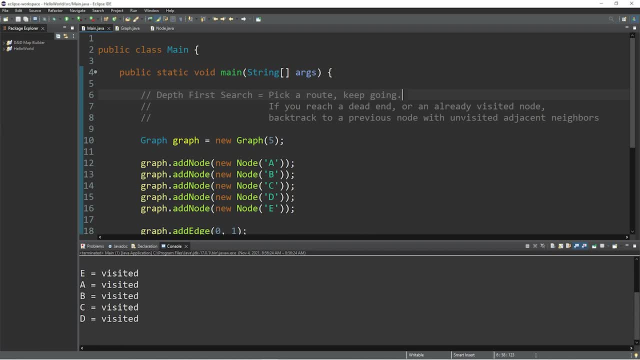 already visited node, you backtrack to the first search algorithm and you pick a route and you backtrack to a previous node with unvisited adjacent neighbors. If you would like a copy of this code, I'll post this to the comment section down below. Don't forget to give this video a 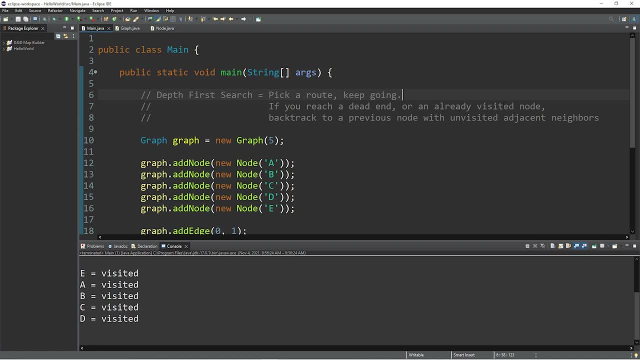 thumbs up, leave a random comment down below and subscribe if you'd like to become a fellow bro. 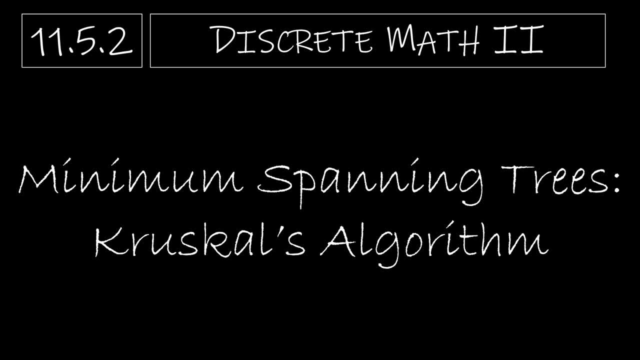 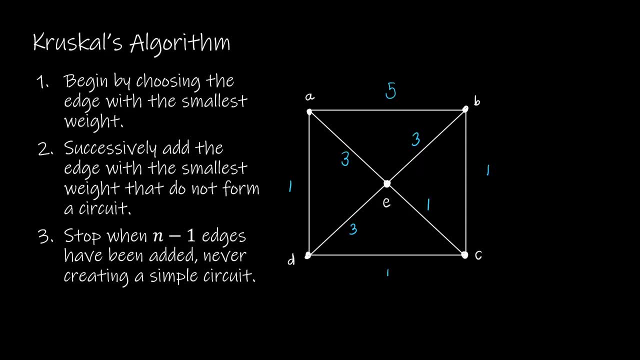 In this video we're going to take a look at Kruskal's algorithm for creating a minimum spanning tree. So for Kruskal's algorithm, we're going to begin by choosing the edge with the smallest weight. So, as you can see on our graph, we 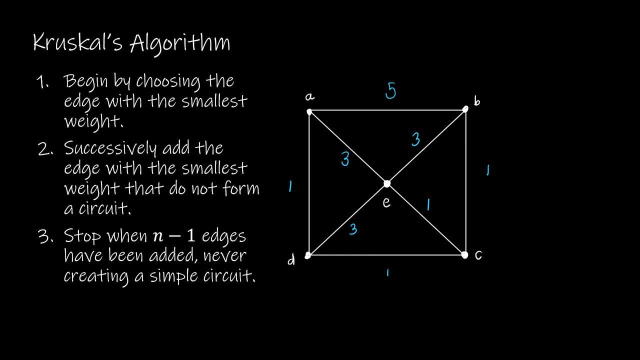 actually have four edges that are of length 1 or weight 1.. So you can choose any one of those, and what we're going to do is continue to add edges with the smallest weight that don't form a circuit. So when we did this with prim, we 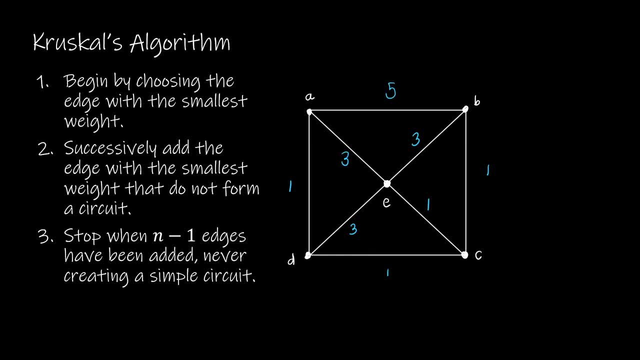 were tied to having to have one vertex that we've already visited connecting to a vertex that we have not. In this case, we are not bound by that. So, for instance, if I want to choose BC because it's a weight of 1, I can do that, and then if I